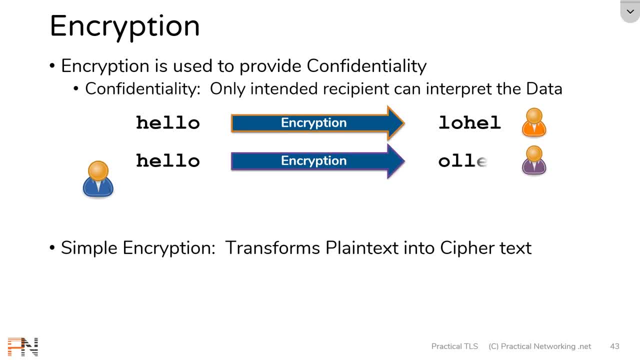 user. the blue user wants to speak to. the blue user is going to have to develop a new transformation. This way, the blue user will know how to turn that back into plain text. The users they are speaking to don't have insight into what was sent on the wire. 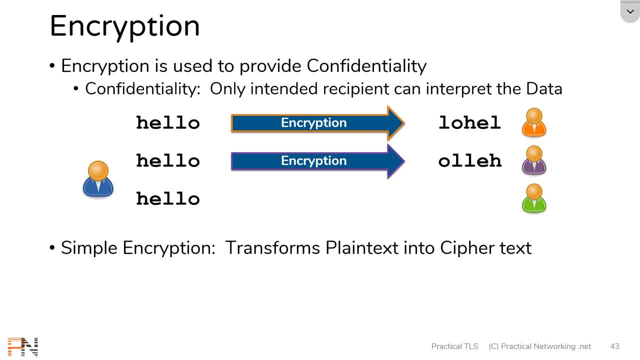 If the blue user wants to speak to yet another person, he's going to have to create yet another algorithm to securely transform the word he's trying to send on the wire. So, as you can see, simple encryption doesn't scale Every user that I have to speak to. I have to. 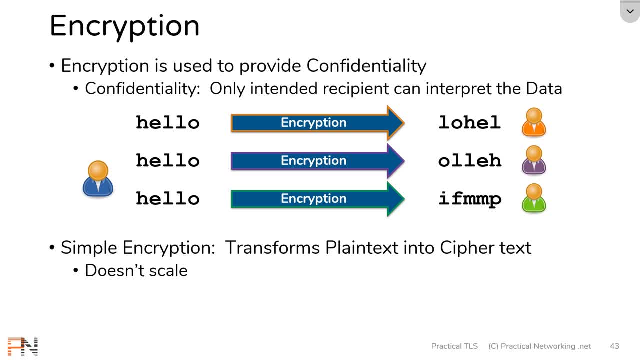 generate a new way of transforming text into something indecipherable- Which, by the way, is very hard to do securely- And that's why I'm going to show you how to do that in this video. It's not a trivial thing to find a way to scramble text to make it uninterpretable by 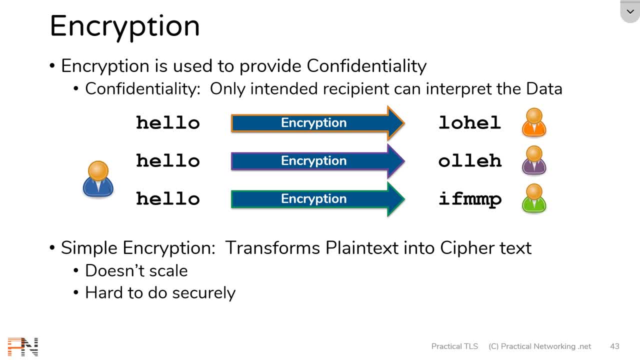 anybody else on the wire. It takes cryptographers and mathematicians years to come up with proper encryption algorithms, And if all I'm doing is simple transformation, I can't just use a publicly known algorithm, because then the entire public knows the mechanism to decrypt. 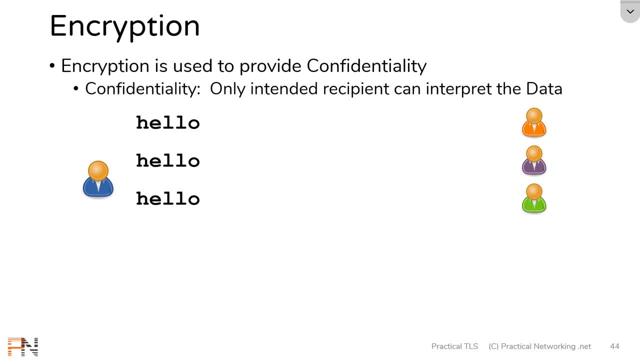 So instead, what the world uses is what's known as key-based encryption. Key-based encryption is going to combine a publicly vetted algorithm with a secret key. The algorithm itself is created by mathematicians and cryptographers and experts in the field. Moreover, it's vetted by each other. 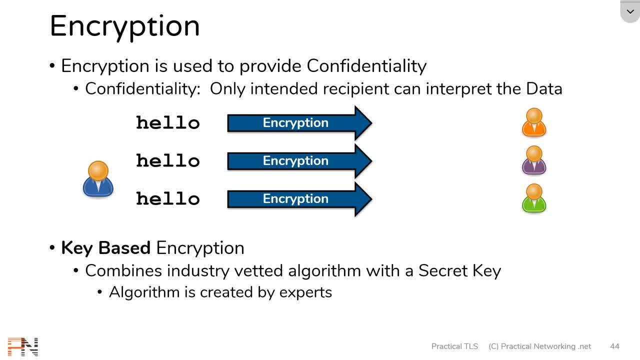 so they actually validate each other's work to make sure that the algorithm are secure. And then the secret key is just a random set of ones and zeros, And even though I'm using the same word to all three of these users and the exact same protocol for all three of these users. 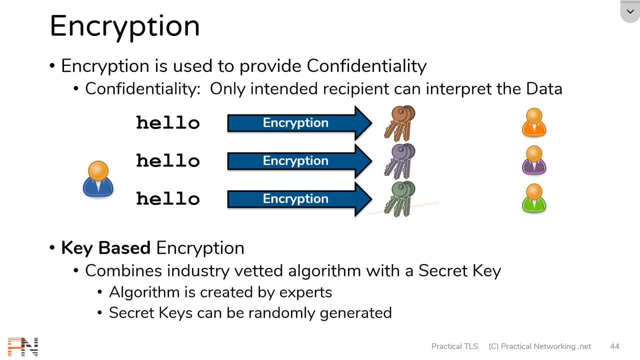 because I've generated randomly new keys for each user on the wire, the ciphertext will look completely unique from one another. This way, the orange user has zero insight into what was encrypted and sent to the purple user, nor does the purple user have any insight into what was sent to the orange user. 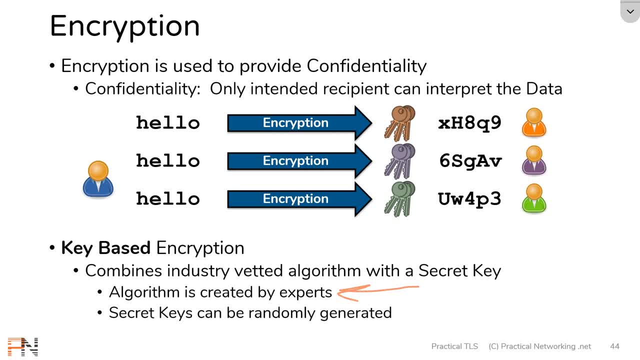 The cool thing about this is I can let the experts do the hard work of creating the algorithm, and it's very easy for me to randomly generate a set of ones and zeros to use as a key. This is what allows encryption to scale to the whole internet. 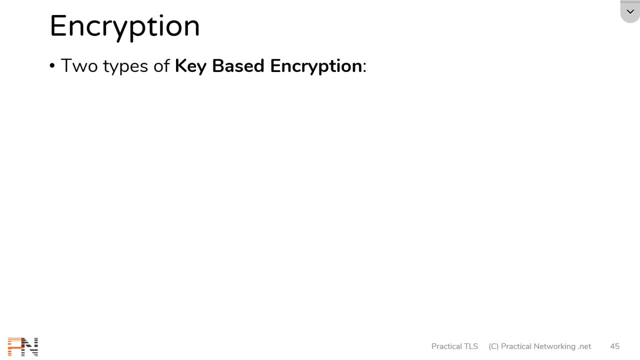 Now there are two ways to do this. The first way is to create a set of ones and zeros. The second way is to create a set of keys. Those two ways are symmetric encryption and asymmetric encryption, and we'll be talking about both of those for the rest of this lesson. 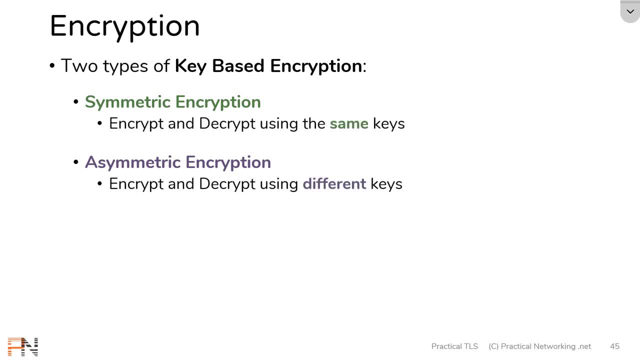 The main difference between these two is that symmetric encryption is going to encrypt and decrypt content using the same keys, and asymmetric encryption is going to encrypt and decrypt using different keys. So let's talk about what that means. To show you how this is going to work, we're going to use the alphabet Now for these examples. 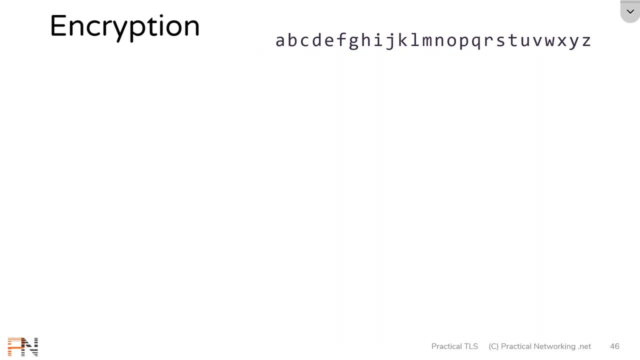 we're going to assume that there's only lowercase a through z, Z. There's no uppercase characters, there's no numbers, there's no symbols. We're going to keep it simple. for the explanation: Symmetric encryption uses the same key for encryption and decryption. 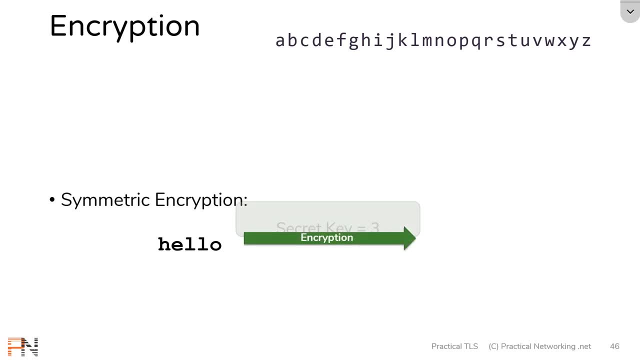 So let's say I start with the word hello. I'm going to use a symmetric encryption algorithm in combination with a secret key. Now, the algorithm I'm going to use for this example is simply moving the letters forward, and I'm going to move it that amount of times. 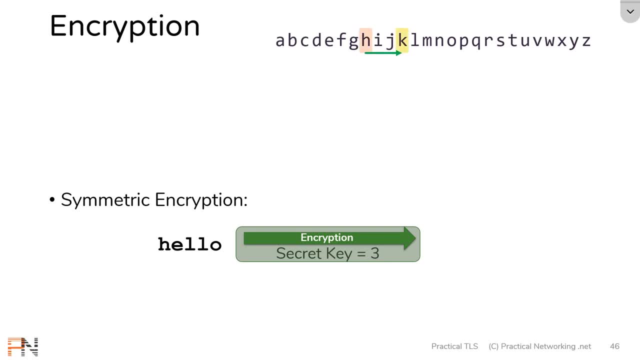 in this case, three. Well, if I start at the H and I move forward three times, I'll end up at K. If I did the same for the rest of the letters in the word, I'd end up with K-H-O-O-R. 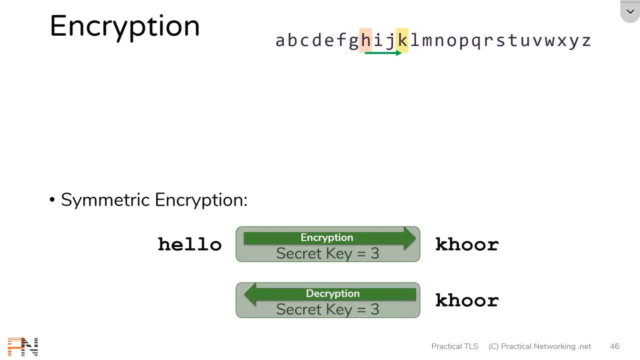 To decrypt this, I would simply take my ciphertext and do the inverse of the algorithm. So if my algorithm was to move forward, my decryption algorithm is going to be to move backwards and I'm going to use the same key. So if I move forward three times to encrypt, 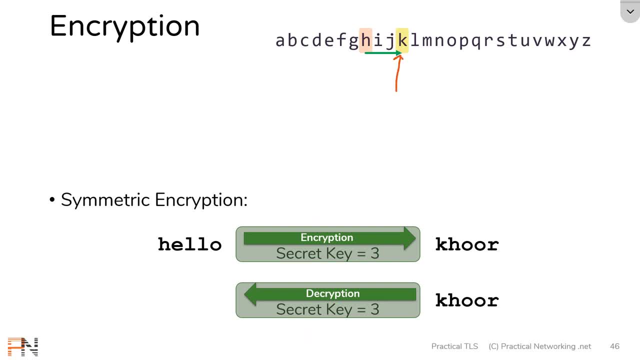 I'm going to move backwards three times to decrypt. If I start at the K and I move backwards three times, I'll end up back at the H, And again I could do this for the rest of the letters to decrypt the whole word. So that's a simple example of symmetric encryption. Notice in: 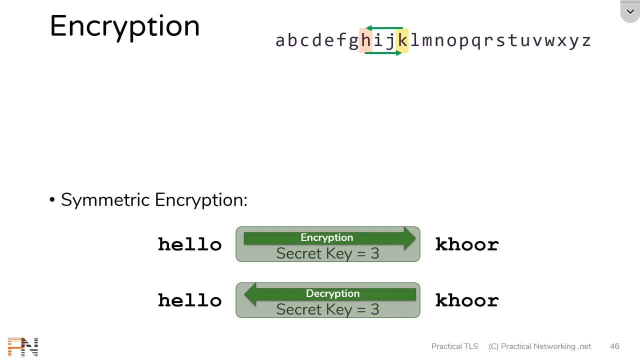 particular, the same key was used for both encryption and decryption. Now let's talk about asymmetric encryption and you're going to see it's a little different With asymmetric encryption. I'm still going to use an encryption algorithm, but the keys I use for encryption and 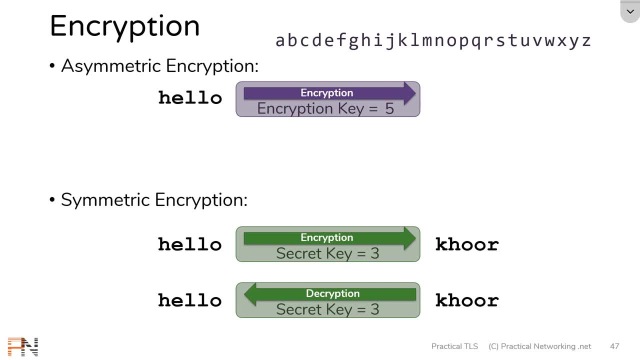 decryption are going to be different. Here. I'm going to use the encryption key of five. Again, I'm going to start with H and I'm going to move forward five times To get to M. I could do it with the rest of the letters in this word to get to MJQQT. 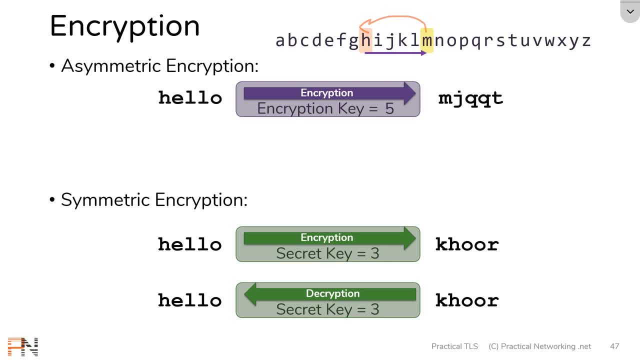 Now it might seem like you can just go backwards to get back to H, but in asymmetric encryption algorithms, the math features what's known as trapdoor algorithms. These are mathematical operations that can only be done in one way. You can't do them backwards. So in the case of 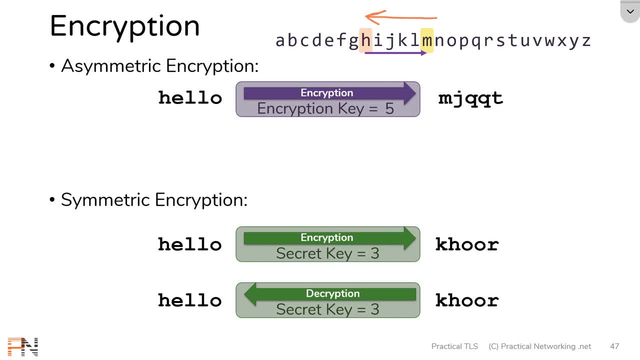 asymmetric encryption. we can't actually go backwards. Instead, we have to go forward a different amount. To decrypt this, I'm going to have to take my ciphertext and use a different key going forward again. So, starting with the M, if I go forward 21 positions, I'll end up back at the H. 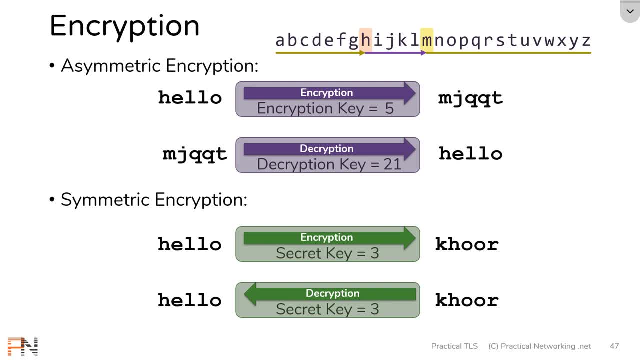 And I could do it again for the rest of the letters, to decrypt, the rest of the word. But notice, I went forward to encrypt and forward again to decrypt, whereas in symmetric encryption you can do forward and backwards And of course with symmetric encryption I was able to use the same key to encrypt and decrypt. 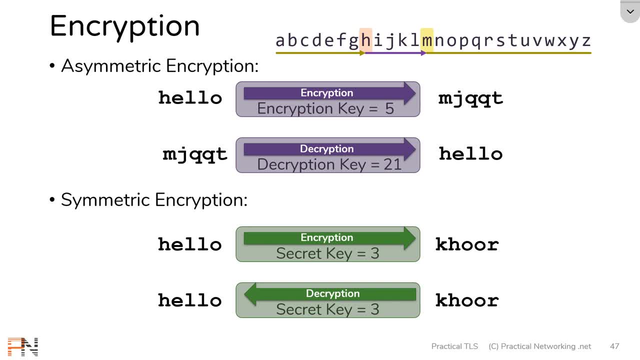 I had to use different keys to encrypt and decrypt. Now let's talk about those keys a little bit more. Those two keys I used in this case, 5 and 21,, are mathematically related. Whatever I encrypted with 5 could only be decrypted with 21.. There are other combinations of keys that you 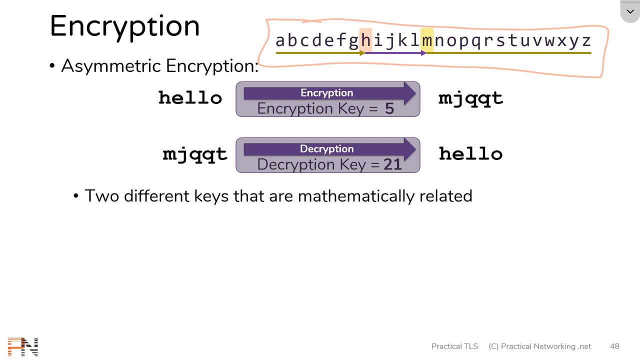 could use in our little example, using just the alphabet. Actually, anything that adds up to 26 would work, So I could have also used an encryption key of 6,, a decryption key of 20, or an encryption key of 10, and a decryption key of 16.. But the interesting thing to note, 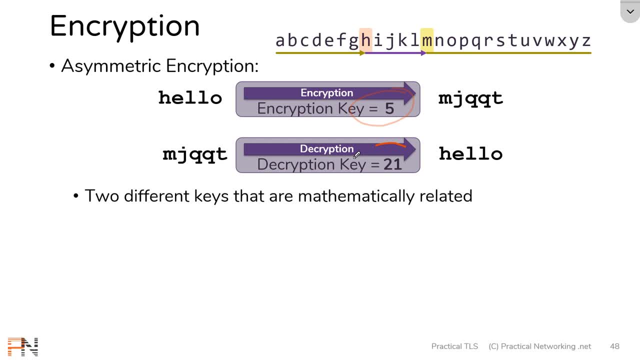 is here. I used an encryption key of 5 and a decryption key of 21.. Well, what if I used them in the reverse order? What if I encrypted with 21? Could I not then decrypt with 5?? Well, let's give it a shot Again. I'm going to start at the H and I'm going to see if I can move forward 21 times. 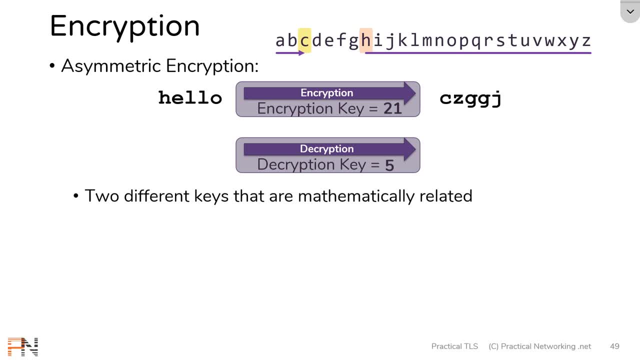 That'll bring me back to the C, and I could also do the same for the rest of the letters, And then, to decrypt this, I would again take my ciphertext and then move forward another 5 times. That would bring my C back to an H, successfully decrypting the first letter of my plaintext. 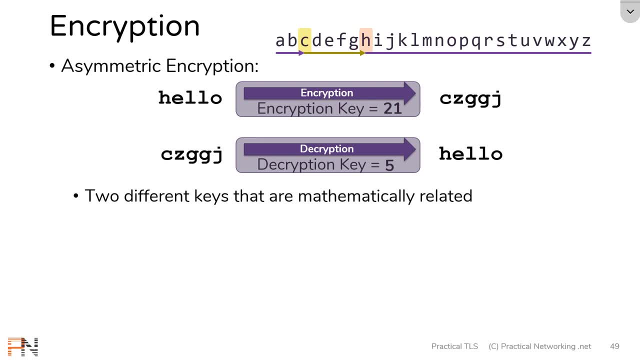 I could again use the same decryption key to decrypt the rest of the letters. The main thing I'm pointing out here is this property of asymmetrical encryption is that you can encrypt with one key, can only be decrypted by the other key, but it works in. either direction. I can encrypt with 21.. I can decrypt with 22.. I can decrypt with 23.. I can decrypt with 24.. I can decrypt with 24.. I can decrypt with 23.. I can decrypt with 28.. I can decrypt with. 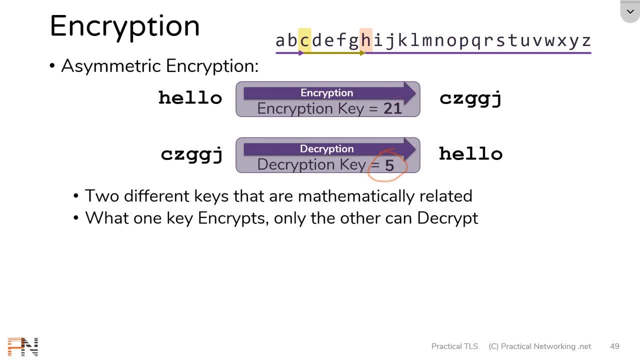 I can encrypt with 21 and decrypt with 5, or, as we showed earlier, I can encrypt with 5 and decrypt with 21.. These two asymmetric keys are mathematically related. Now, what the industry does with this is they take one key and they label it as the public key and they make it available to anybody that. 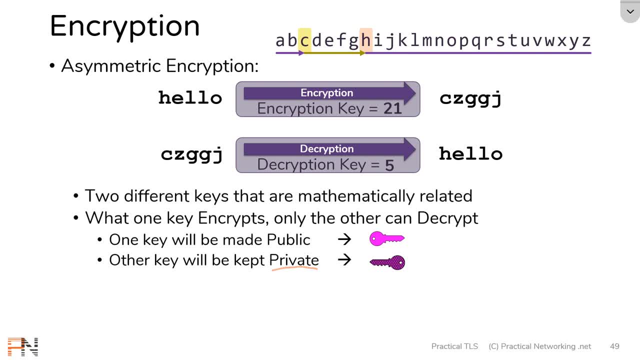 asks for it, And then they take the other key and they call it the private key and they keep it to themselves. They never share their private key with anybody else. This way, anybody can use your public key to encrypt something, but only you possess the private key that allows you to decrypt. 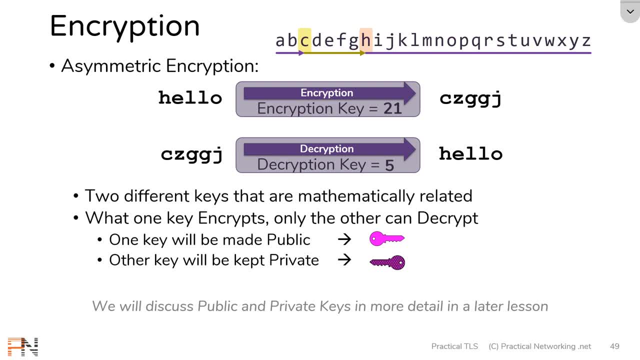 it Now. we're going to be talking about public and private keys in more detail. in the next lesson We're going to show you the different operations you can do with public and private keys, But for now I want to continue comparing and contrasting symmetric and asymmetric encryption. 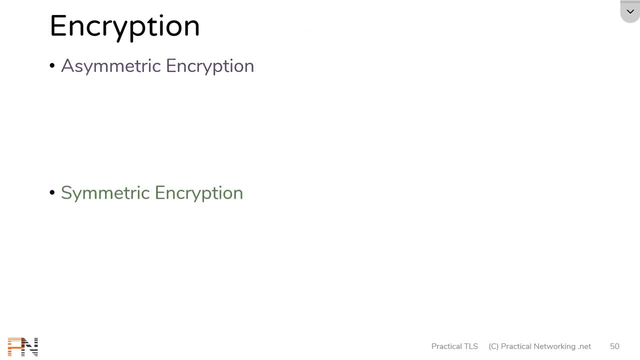 Next, I want to tell you about the strengths and weaknesses of either method of key-based encryption. Now you'll notice that these strengths and weaknesses are in relation to each other. The first one we're going to talk about is that symmetric encryption is a method of key-based encryption. Now you'll notice that these strengths and weaknesses are. 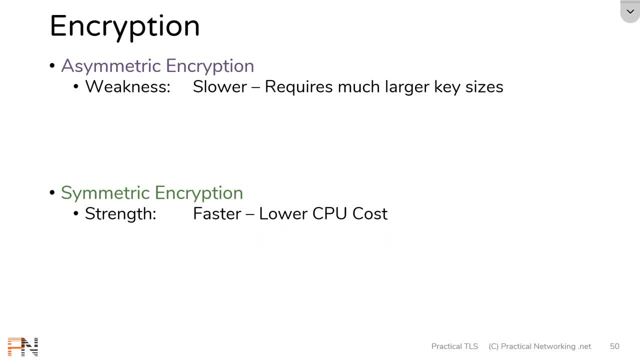 faster. It's easier for CPU to do the math and work with the keys of symmetric encryption algorithms, Whereas asymmetric encryption is slower. It is harder math and uses bigger keys. Therefore, when comparing the speed of asymmetric encryption and symmetric encryption, symmetric encryption is much faster. Moreover, symmetric encryption has this: 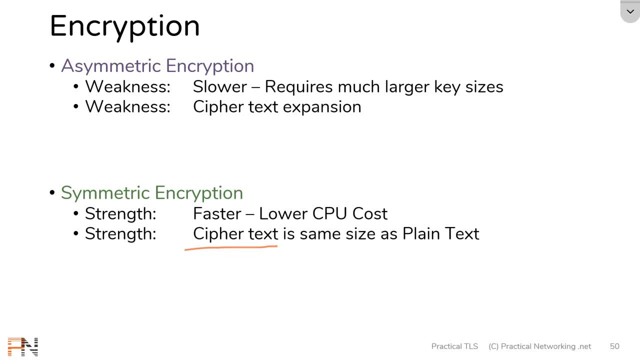 interesting property that the ciphertext that you've encrypted ends up being approximately the same size as the plaintext. The benefit to that is that when you put something through an encryption algorithm, that doesn't end up doubling or tripling the amount of data you have to put on the wire. Asymmetric encryption has the unfortunate 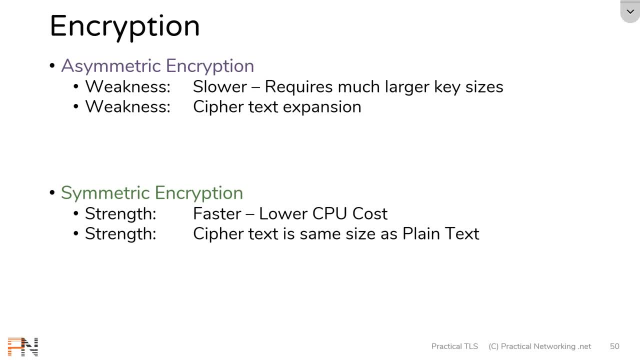 property called ciphertext expansion, where typically what you end up encrypting with asymmetric encryption ends up being larger, size-wise, to what you initially had as your plaintext. And finally, a weakness of symmetric encryption is that, since you're using the same key on both sides, that secret key must be shared. That's a problem because you have to figure out. 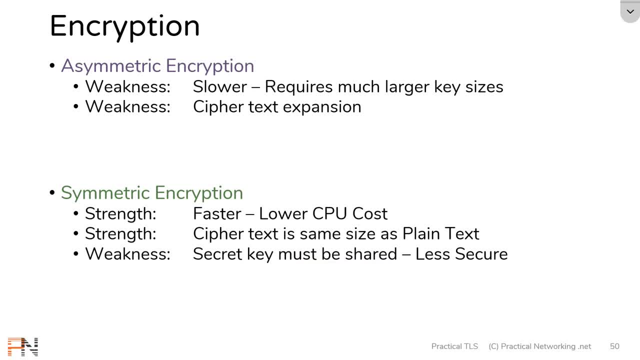 how do we get the same key on either sides of the wire in a secure way? Therefore, symmetric encryption is considered less secure than its asymmetric counterpart. With asymmetric encryption, that private key never has to be shared. You never need to send that to anybody else. Therefore, since that key never needs to be shared, it ends up being more. 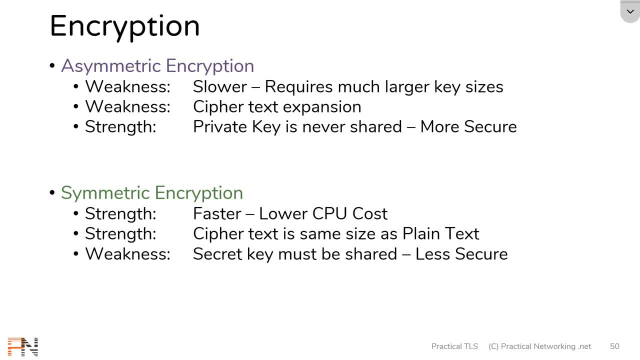 secure than its symmetric counterpart. Now, these strengths and weaknesses make symmetric encryption and asymmetric encryption ideal for different usages. Symmetric encryption is ideally used for bulk data protection, That is, if you want to send a bunch of data from one party to the other, you want to use symmetric. 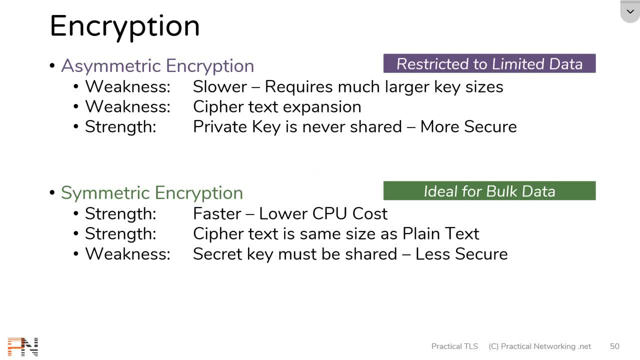 encryption: It's faster, it's more efficient, but unfortunately you have the problem that it is a little bit less secure. If, however, you only need to send a smaller data set, then go ahead and use asymmetric encryption, because it's more secure And since you're 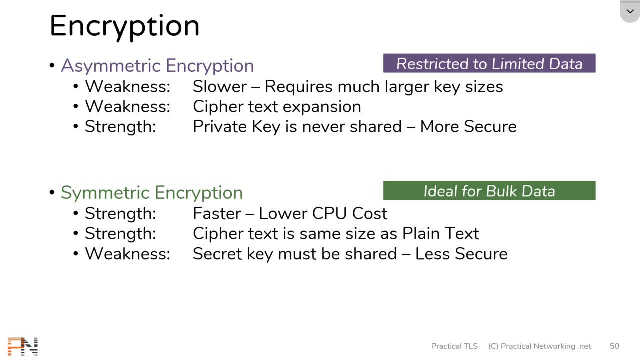 only using a smaller data set, you're not taking that big of a hit insofar as its slowness or the ciphertext expansion. So keep these strengths and weaknesses in mind, because in the next lesson I'm going to show you how we use the strengths of one to compensate for the weaknesses of the other. 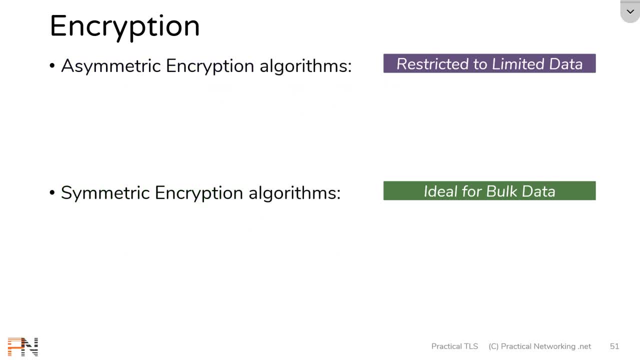 Otherwise, the last thing I want to show you in this lesson is just a few asymmetric and symmetric encryption algorithms, just so you know which are which. This list is a bunch of asymmetric encryption algorithms: DSA, RSA, Diffie-Hellman, Elliptic Curve, DSA and Elliptic Curve, Diffie-Hellman. 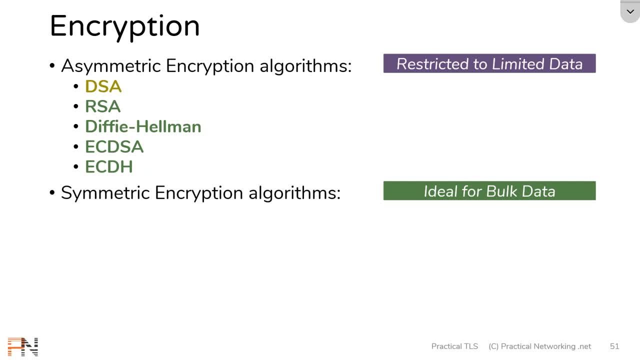 Those are all asymmetric encryption, which means they are more taxing on CPUs and involve values known as public keys and private keys. And these are a list of symmetric encryption algorithms, which means they are less taxing on CPUs and require the same secret key on either side of 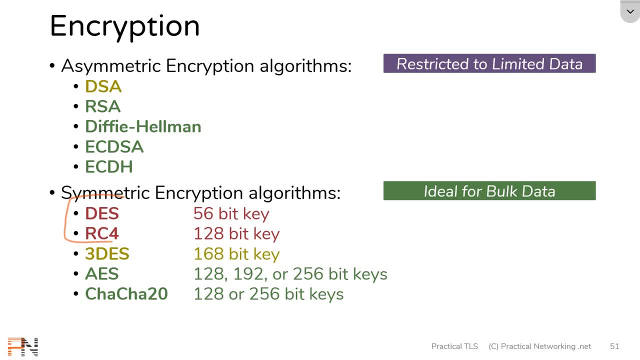 the wire. Now notice DES and RC4 are in red. That's because these algorithms have been considered completely insecure by today's standards. Generally with symmetric encryption algorithms, the bigger the key size, the more secure the algorithm. This isn't always the case. Notice triple DES over here has an advertised key strength of 168 bits.